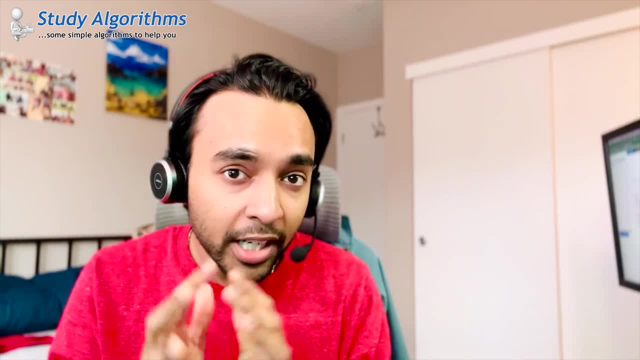 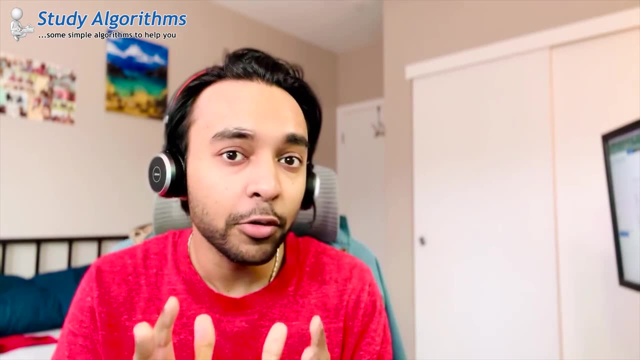 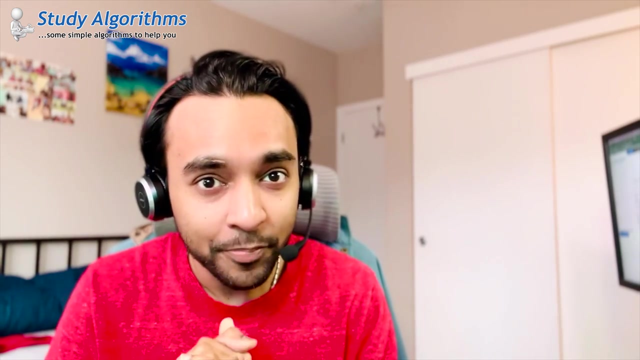 the recursion based algorithmic paradigm. So to get a quick recap of brute force and recursion, find the links in the description below to my previous videos. I highly recommend you to take a look at them Because if those concepts are clear to you, you will understand backtracking really quickly. 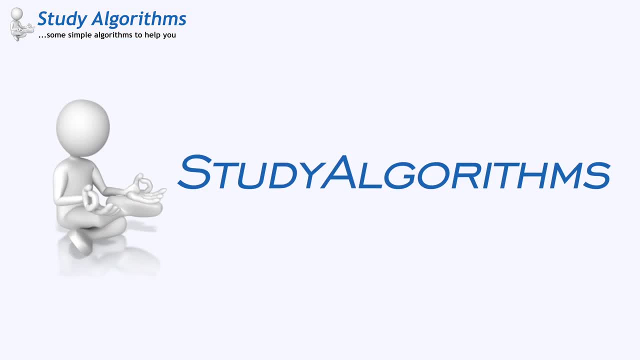 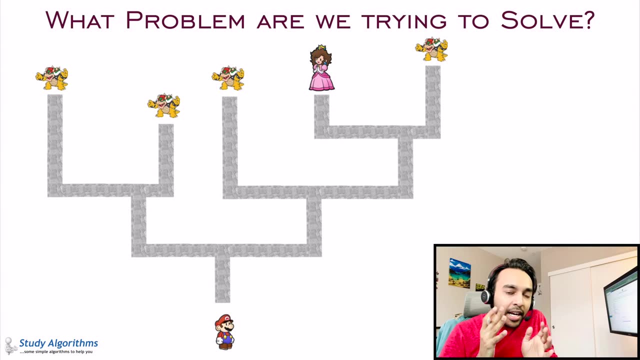 So if you're ready, let's get started. I always believe that when you're trying to learn a new concept, it becomes very easy if you can relate it to some real life example. So, going back to our example of video game, I have this kind of a scenario in front of me, right? 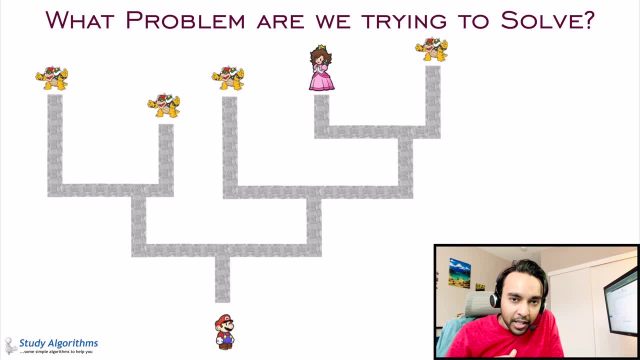 And I am playing a video game With my character, Mario. you all must be familiar about Mario, right? So while you're playing the game, this is a kind of situation where you come across, you have Mario and then you have so many paths in front of you And if you realize that only one of the path will 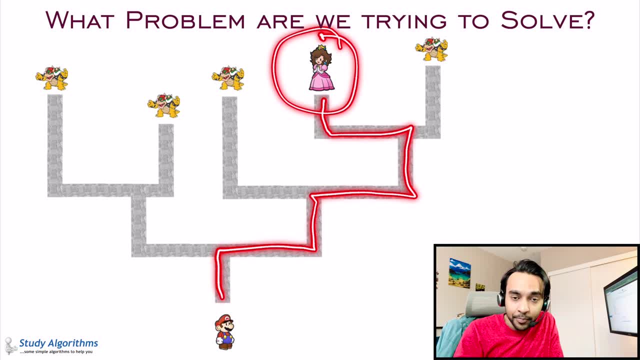 lead you to Princess Peach, where you want to go correct. All the other paths will lead you to King Koopa, who is destined to kill you, right? So what do you do? How do you find this path? So this is the problem that you have at hand, And now you have to start thinking: what can? 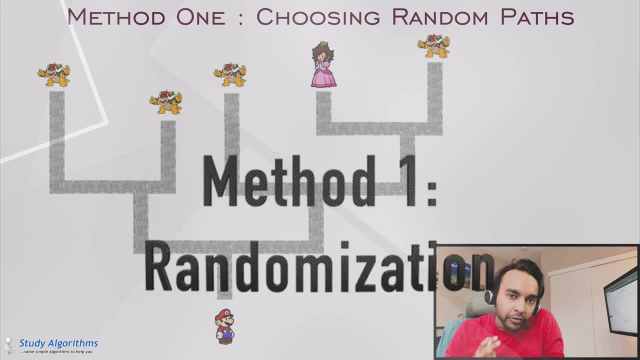 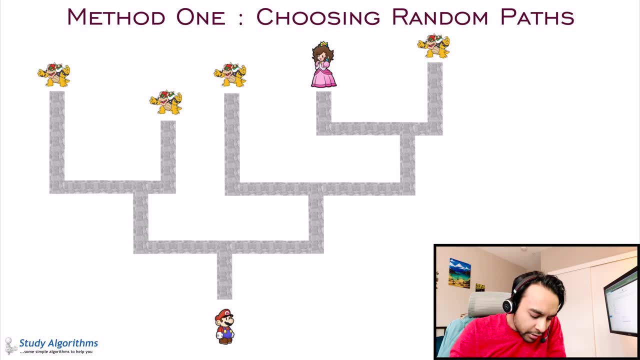 you do about it. So one of the ways that you can start to approach this problem is by selecting any random path that comes to your mind. So what you can do is you can take your character, Mario, and you take him one step up. You now have to take a decision between either going to the right 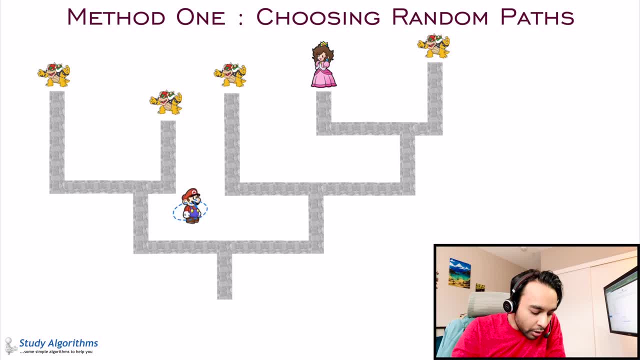 or going to the left. Correct. Randomly, you decide: okay, I will go left, And then you move ahead Once again. you have two paths And this time you say: you go right. If you go right, you encounter King Koopa. 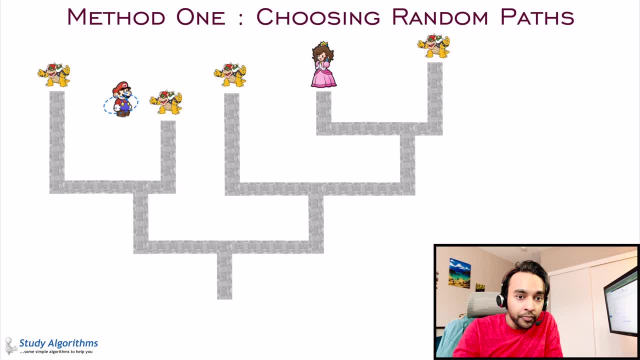 Oh my God, So this is not the correct path, right? So what you can do is you can try to come up with an alternative path Once again. you can do this randomly. You will take Mario and okay, last time you went left. Okay, So this time you can go. right, I go right this. 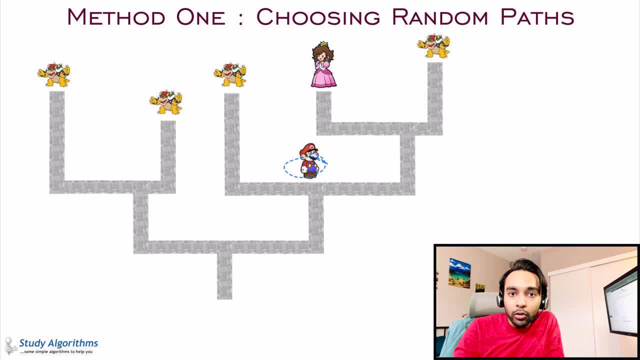 time, Okay. So this time you can see again. I move ahead again, and what do I do again? Let's say I go right again, and I'm again having two places to go: Left or right. This time let's say I go left, Okay, And voila, I met my princess. So the game ends, Correct. But 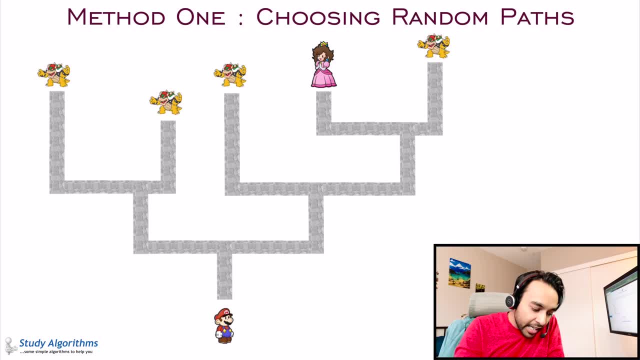 it could also have been possible that when you were taking your character, Mario, at certain places you could have gone right, and then right again, and then right again and again King Koopa. So you go back again, And what, if you went left this time, You might have. 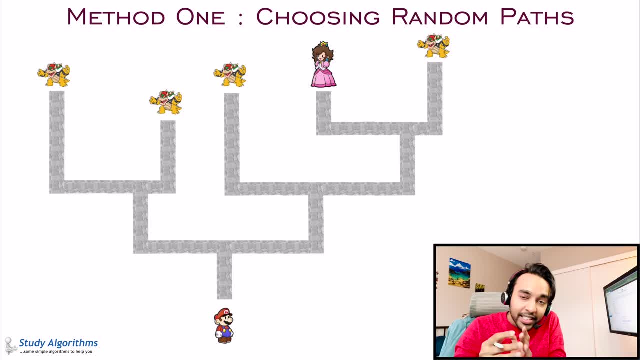 again met King Koopa. So this is a kind of a random approach And sure, if you keep on taking random chances at every time, what will happen is, eventually you will find a path where you will meet your princess, Correct. But there is no certain way where you can. 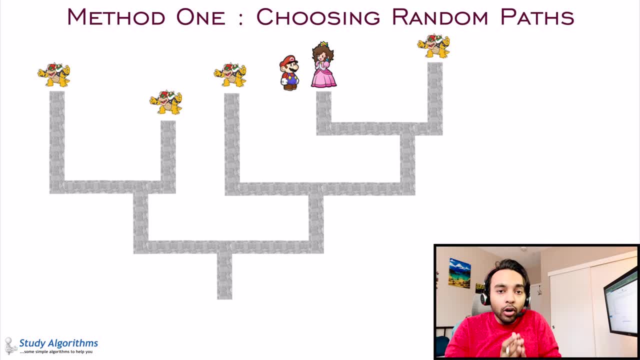 determine. okay, this is the method I am going to take, or this is the way that I'm going to take to reach my princess. So what you were doing up till now, you were trying to approach this problem in a brute force way, That is, you are trying every possible combination. 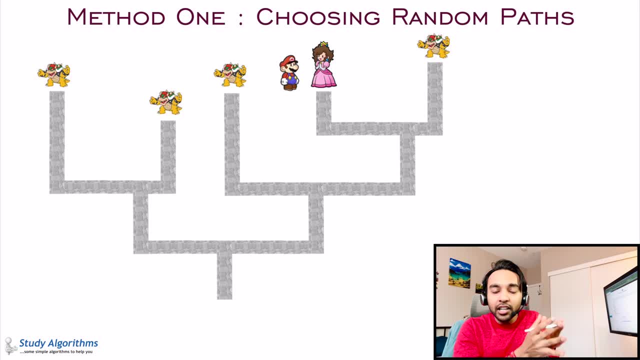 just to get at your princess, just to arrive at your answer, Right. So this approach is not efficient. The problem you are facing is that, whenever you start a path you do not want to reach your princess, You want to reach your princess. You want to reach. 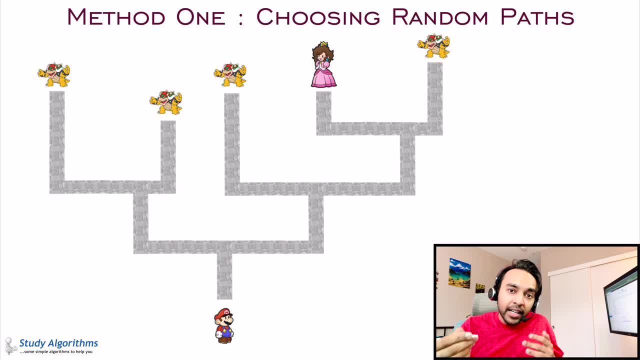 your princess. You do not know whether you have to go left or you have to go right, And the next time, whenever you are encountering the same position, you do not know if you have already went towards the left or not. Correct, So how do you solve this problem? 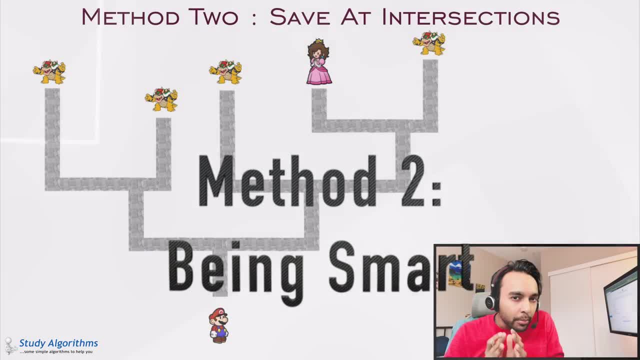 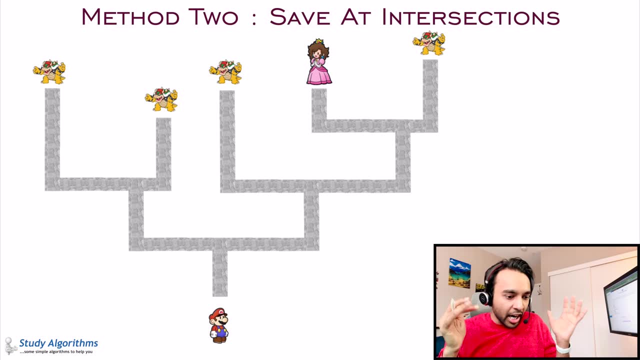 If you play video games a lot, one thing that could come to your mind is: you can save your game at several instances, Right, So you can try to form a strategy in your mind. What you can do is, after Mario bounces, at any point where you are having two choices: what? 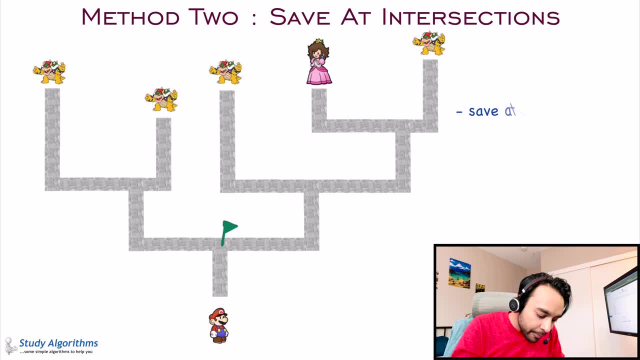 you can do is you can save your game at that point, Right, And then what you can decide is: at every intersection, I will take the left path first. So what I'm going to do is, after saving my game, I go to the left direction. Right Now, my Mario is at this position, Correct? 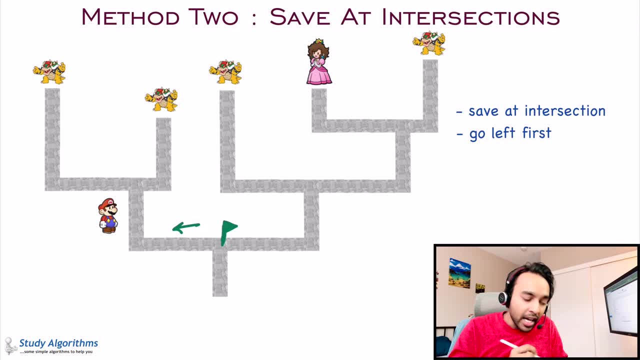 Once again, what you see is after Mario bounces. at any point where you are having two choices, you have an intersection, And how do you decide where to go? Once again, you will save your game over here and you will go to the left direction. Right Now, Mario moves ahead. 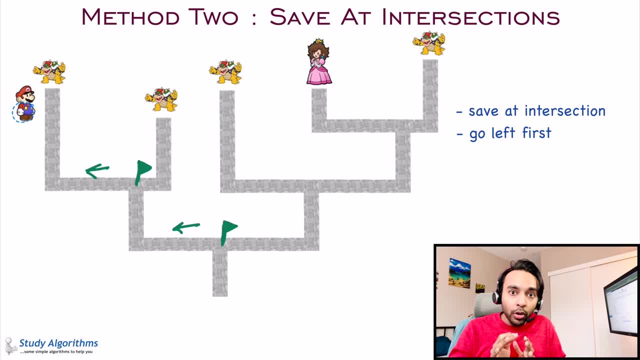 in this path and reaches King Koopa. So you realize, hey, this is not a correct path. So, instead of going back all the way to the starting and then trying out new positions, what you're going to do is you will take Mario and move it to the last saved. 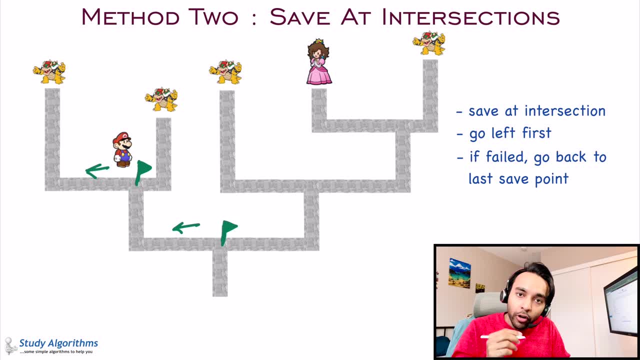 position that you have Right. And this time what you can do is you can go to the right direction. If you go in the right, you will again see that, hey, I found King Koopa. So you have eliminated both of these paths, Correct, And this is not the right way to go, So what? 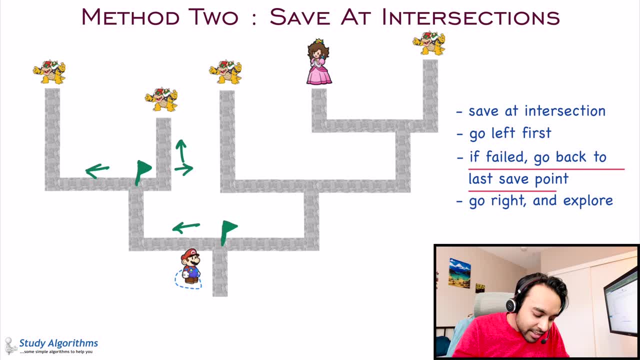 you're going to do next is you will go back to your last saved point, And this is this point. Right, You have now covered the entire path in the left. You know that this is the starting point. You know that nothing exists over there. Correct Similarly what you. 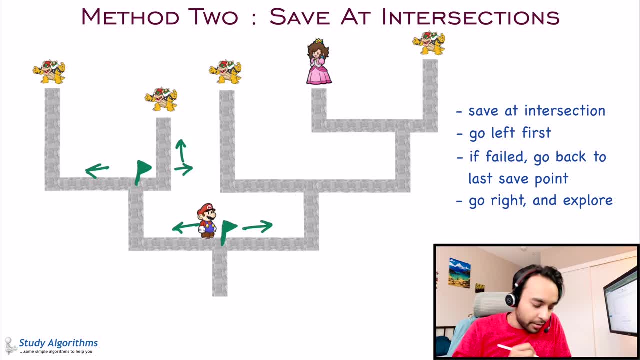 can do is now you can start traversing in the right direction. So Mario will start moving to the right And once again he sees an intersection. So what you're going to do, you will once again save your game at this flag And then first go to the left direction, Because you have 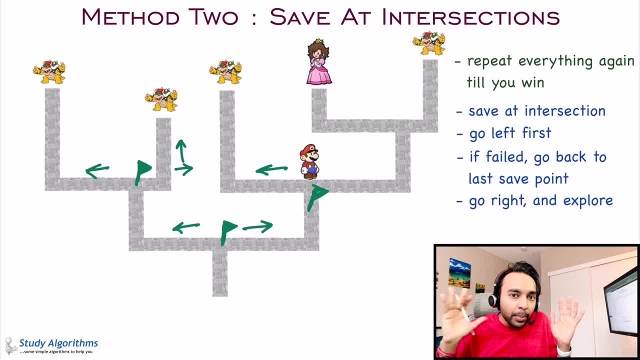 to follow a certain pattern. That is how you can keep a track of all the stages Or all the positions you have been in. So now Mario goes to the left and he encounters King Koopa again. So now you know this is also not the correct path And, once again, 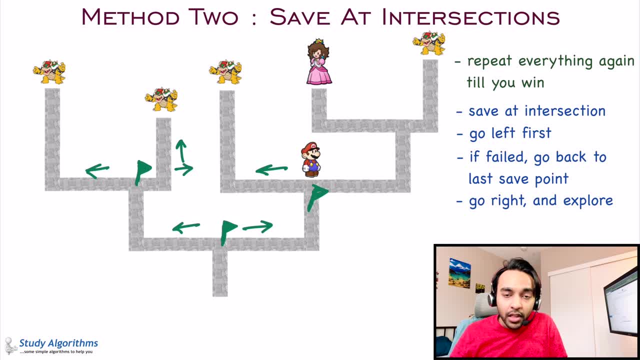 you can bring back Mario to your last save point. So now, what do you do? You know you have covered the left path, but there is also a right path. So you go in the right direction And once again Mario is at an intersection. What do you do now? You will go to the left. 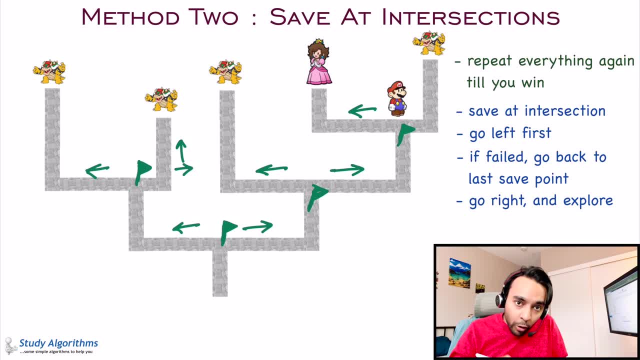 path and save this path. Save this point Correct. Now, when you move to the left, you will hop on this path and ultimately you found your princess, right, And Viola. your level is over, So you beat the game, Correct. So what were you doing at every point? At each of these points, you 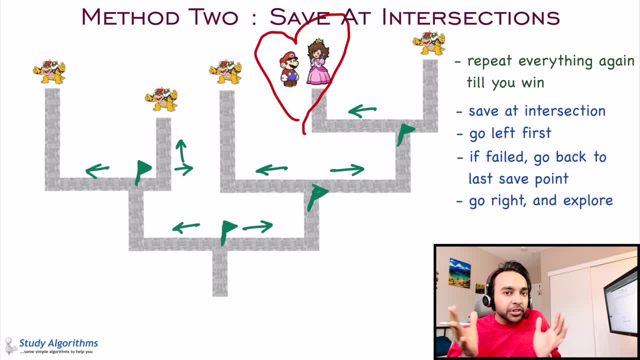 were trying to look at the state of all the positions. you have been in Correct And this is the way the backtracking algorithms work. So now you can see that you have found your princess And Viola. your level is over, So. 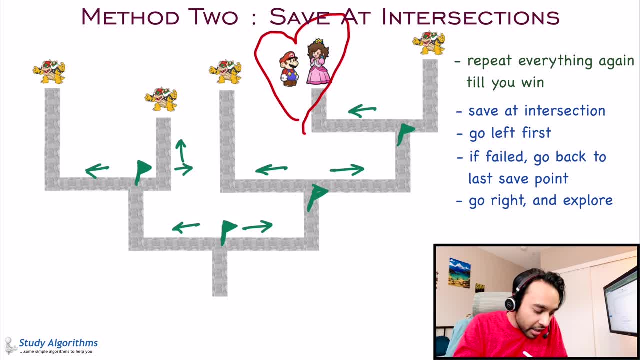 you beat the game Correct. So what were you doing at every point? At each of these points, you are looking for backtracking algorithms. What were you actually doing over here? When Mario was at this point, he saw that there is Kinkuba. So what do you do? You backtrack. 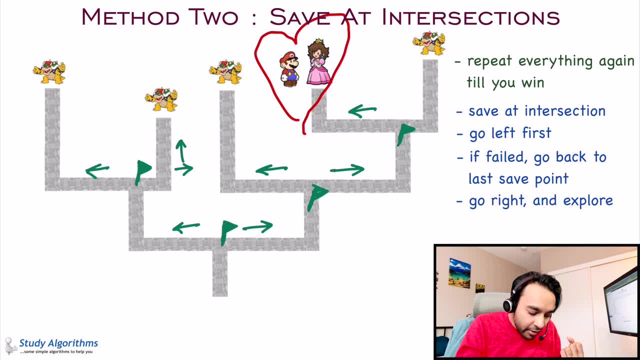 to the last state And then you use the last and other paths. you then backtrack from this state. you will try to discover new possibilities. If this entire state does not get to your solution, you will backtrack again and go back to the last state that you found. This was the last. 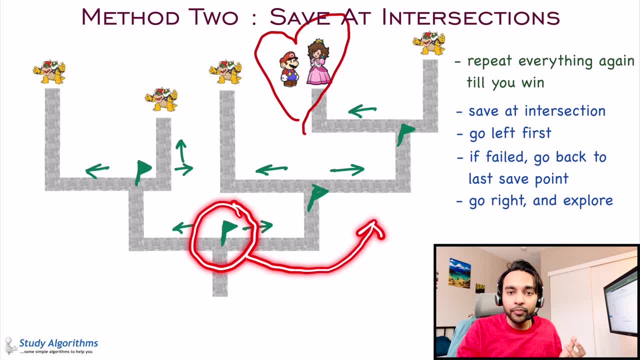 state right Thirty-four, There was someone called Erich Ruysag. Each of thesemondays, one of your start proceeding in the other direction. So this is how backtracking works: You go ahead and explore a state. If that will not give you the solution, you come back. That is. 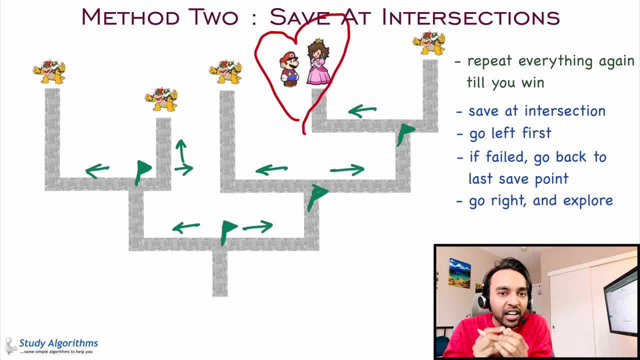 you will backtrack right. That is why the name backtracking algorithmic paradigm. So at every moment you try to go out and explore a space And if that does not work out, you go back to your original state or you backtrack. So this is how the backtracking algorithm. 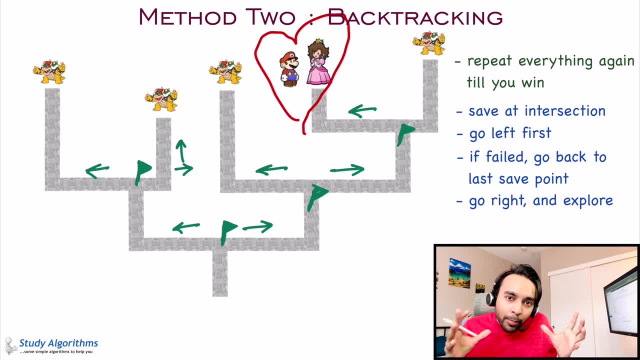 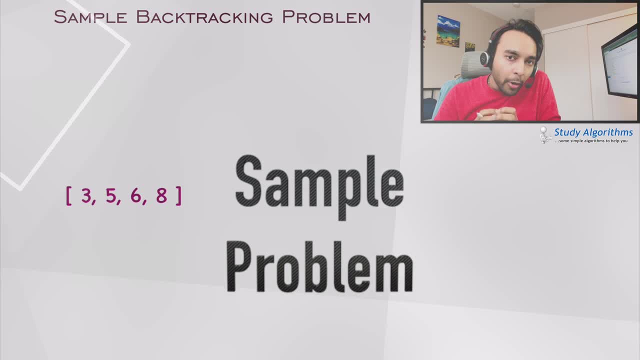 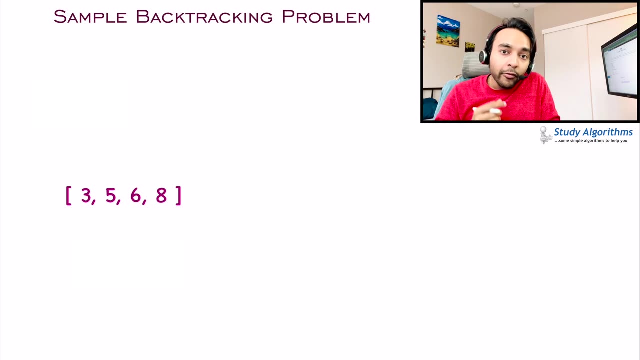 works Pretty simple, right, And based upon this approach, you can start to solve some of the programming problems. One of the very popular programming problems that is based on backtracking would be finding all the subsets of a given array. What is a subset? A subset? 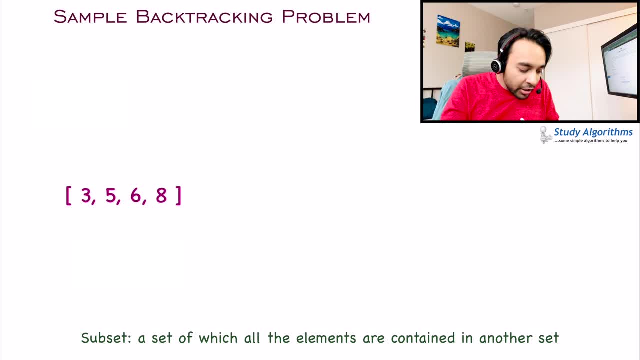 is any smaller set that can be formed using any of these elements from this original set. So, for this example, all of these can be your subsets. Sure, There will be other subsets as well, and they would be so many right. So how does backtracking work in that context? To take up a simple example, let us just take 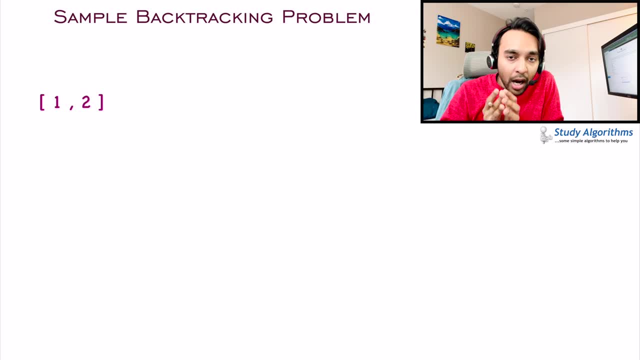 an array that has just two elements. So now I ask you, okay, tell me all the possible subsets of this array, how you can go about doing this using the backtracking approach. So first of all, what I'm going to do is I will just make an empty set, right, Because? 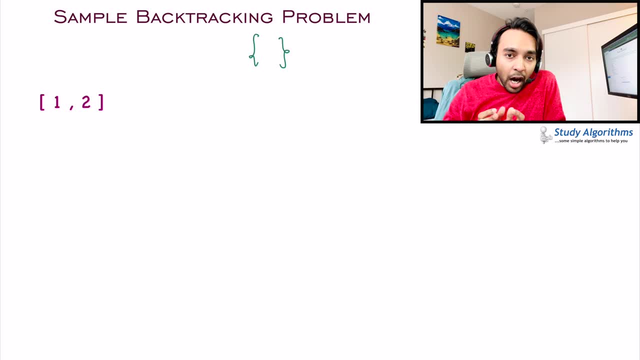 an empty set is also a subset. right Now, what can you do? Remember, Mario, where at each state, you had two choices right. So what you can do is you can look at the elements of this array and now you can start with the first element and decide: should I make? 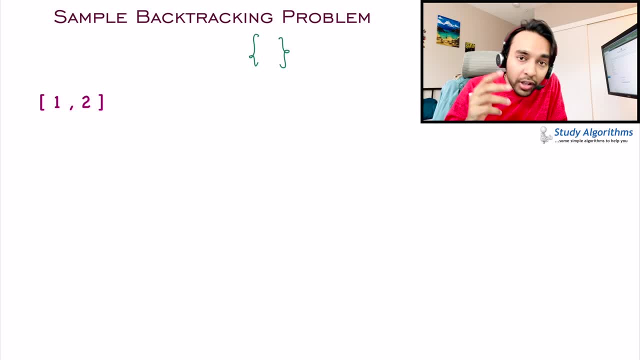 this element. Do you want to take this element or no? So this is similar as the left and right choice, correct? So either you take the element one or you do not take the element. If I'm taking the element, my subset becomes like one, And if I do not take the element, 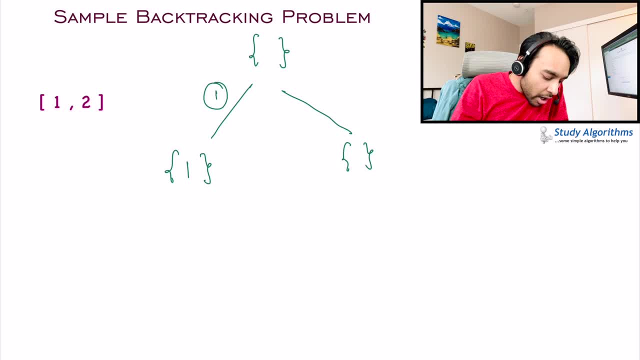 my subset still remains empty, right. So now I have completed my operation. with the element one Going forward, I have my next element two. Once again, I have a choice: do I want to take the element two or do I not want to take? 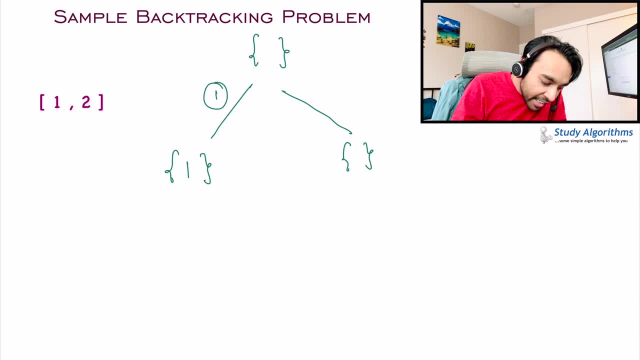 the element two. So what I'm going to do is, at each of these states, I will just try. okay, I am taking the element two and I do not take the element two. And for the other state also, I take the element two and I do not take the element two. So these will give. 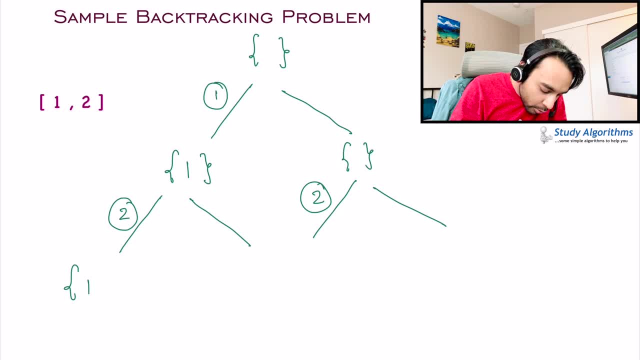 me new sets. So when I take the element two, I get one set. and when I take the element two, I get my subset as one comma two. If I do not take two, I just get my original subset. Now in the next state, if I take the element two, then my set becomes two, And if I do not take 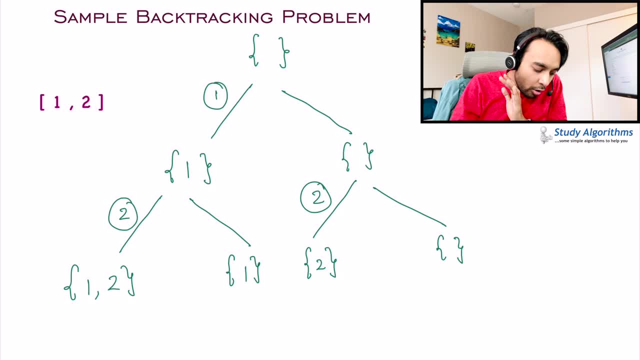 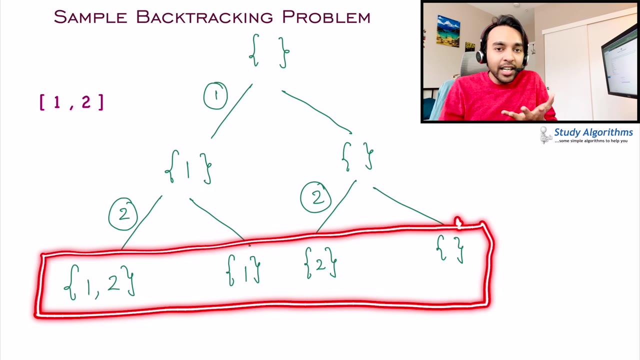 the set remains empty. So now you see all of my elements have exhausted. right, And if I look closely, these are all the subsets that are possible. right, You cannot form any other subset. What is different from these? Certainly, you cannot duplicate the elements. right Talking. 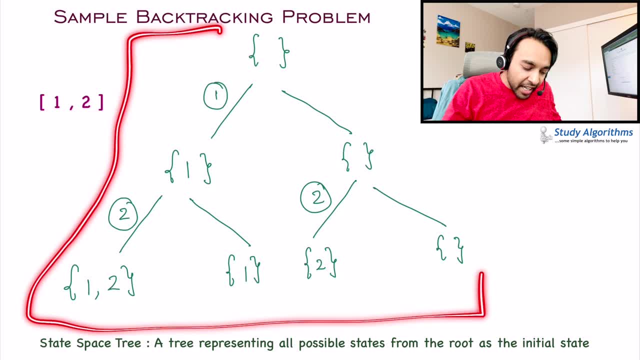 about some technical terms. this is known as the state space tree. That means it is defining every state your set could be in. So this is a single state, This is a state, This is a state And this is a state. You have to find out all the unique states and 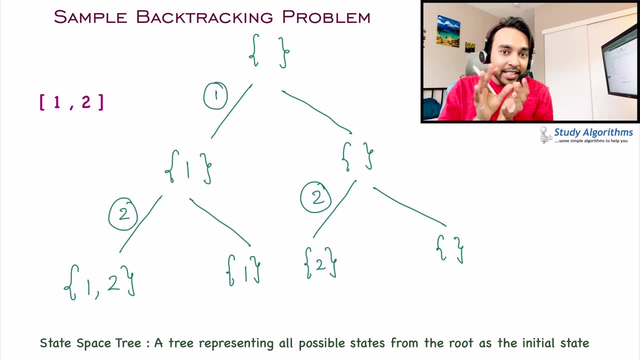 this would be your answer. So this state space diagram represents all the states that are possible. This state space diagram depends upon the type of problem you are solving. A very complex problem could have a very huge state space diagram. That means a lot of possible cases. 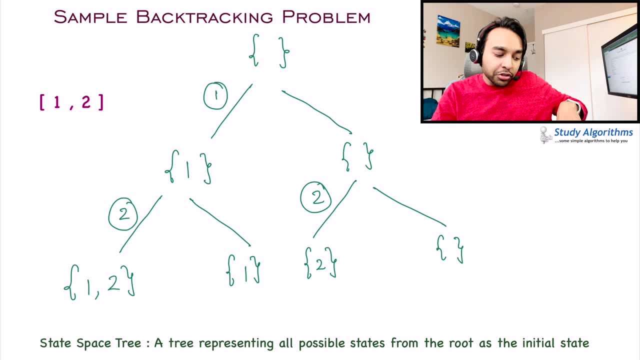 Think about when you're playing a game of chess. If you're trying to solve chess using backtracking approach, what will happen? Suppose you have a rook. That rook can move in any of the directions right And for each of the direction you will have a different state. 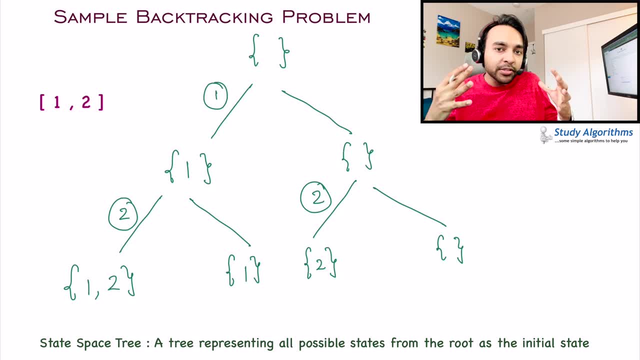 space tree. So chess is a very complex problem. It is a very complex problem. It is a very complex problem. Chess is a very complex problem that can be solved using the backtracking approach, but that will come later on. Right now, I just want you to get a feel of the backtracking. 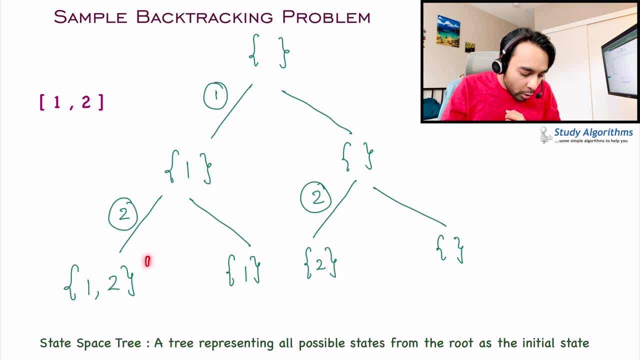 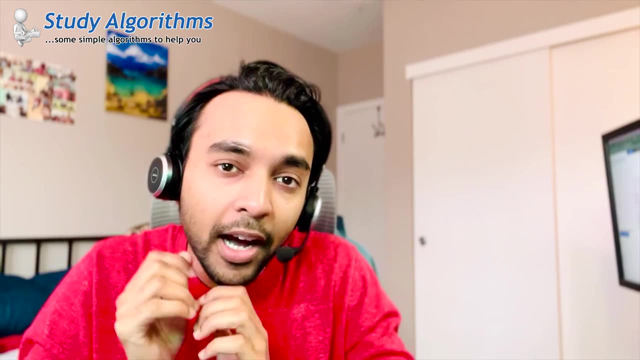 approach. How does it look? Basically, you just go at a state and then backtrack to find other states. right, And this is all how a backtracking approach looks like. We will look at the code for this problem in one of my later videos. I hope I was able to simplify. 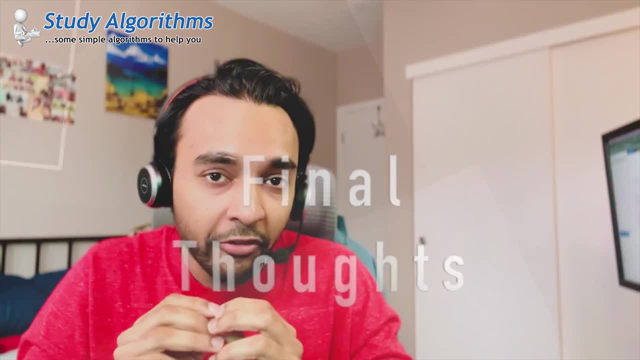 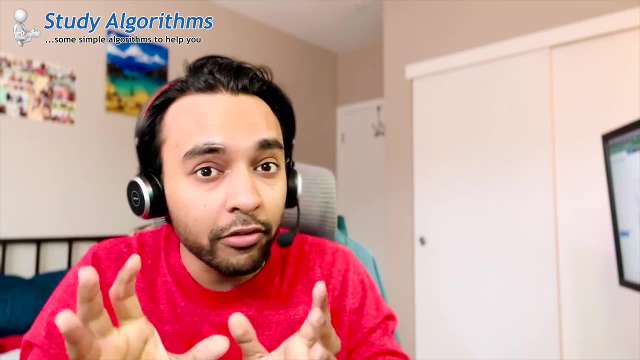 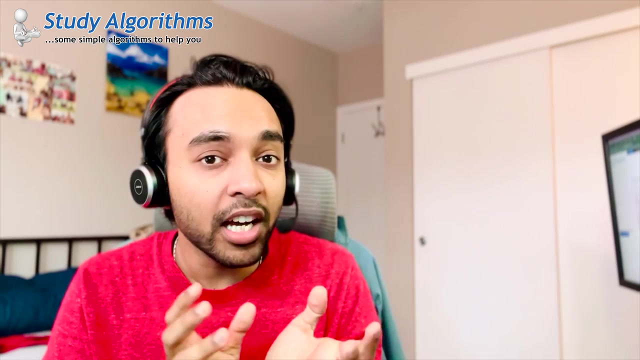 the backtracking algorithmic paradigm for you, As per my final thoughts. take a moment to think which are the specific kind of problems which can be approached or solved using this backtracking algorithmic paradigm, For example. I will give you a hint. Think about puzzles, Think about some problems where you are given. 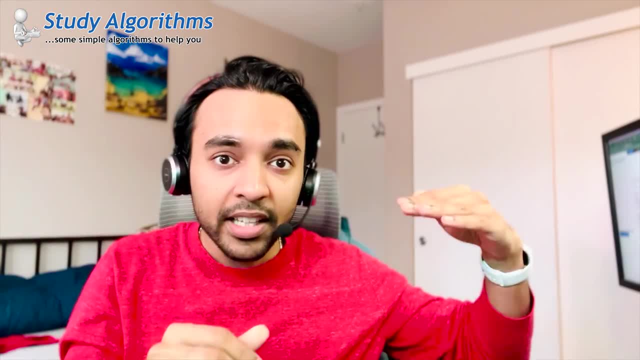 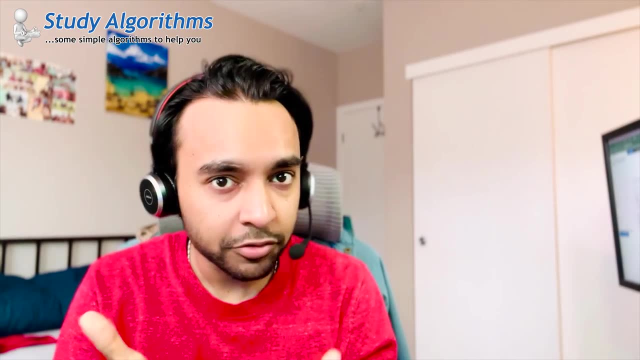 a maze and you have a start point and an end point, Then you have to navigate your path, come back to the previous path and then find a new path right. Similar is the case with Sudoku. If you are solving a Sudoku, then if one of the choices do not work, you will. 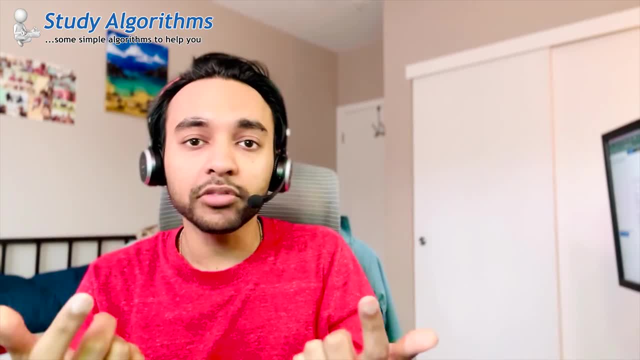 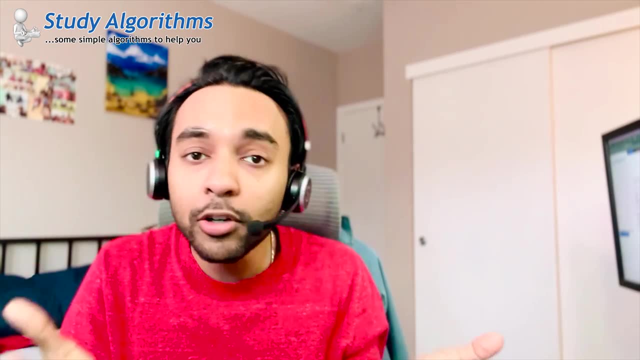 try to change the number and then come back again with new choices, right? So these are all examples of backtracking. Which other problems did you face where you were able to apply backtracking? Tell me other examples that you found out. What problems did you? 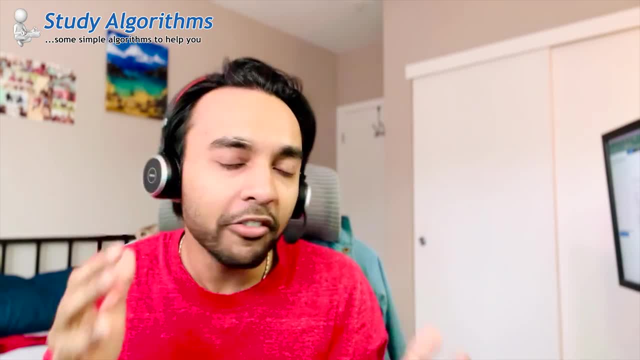 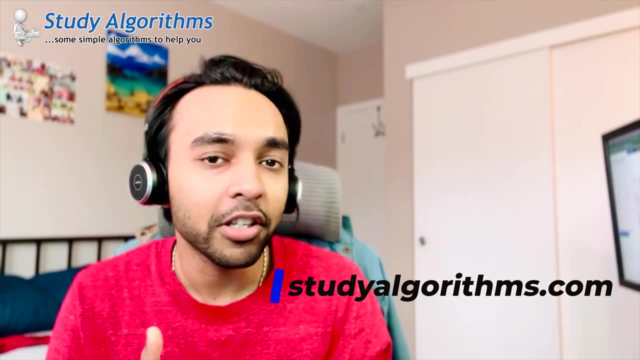 face. I want to know everything in the comment section below and I would love to discuss all of them with you. You would be also glad to know that a text-based explanation to this content is also available on the website studyalgorithmscom- a pretty handy website.